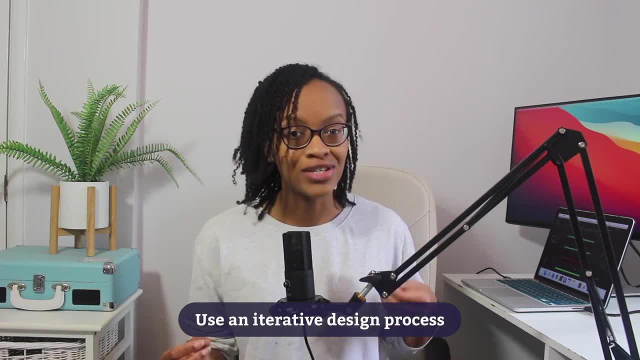 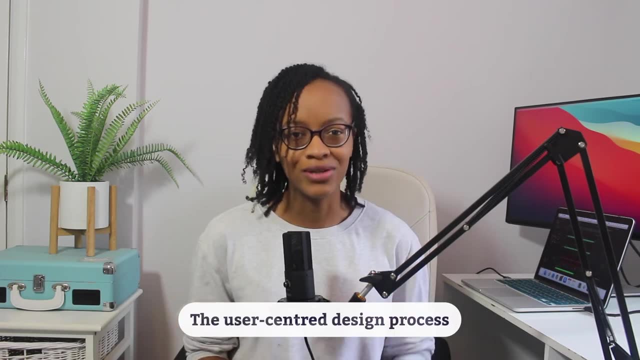 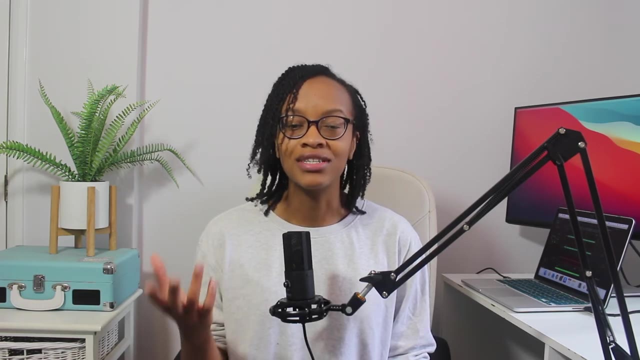 user-focused decisions, Use an iterative design process. Speaking of iteration, this brings me nicely onto the user-centred design process. As mentioned earlier, user-centred design is an iterative design process in which designers focus on the users and their needs in each 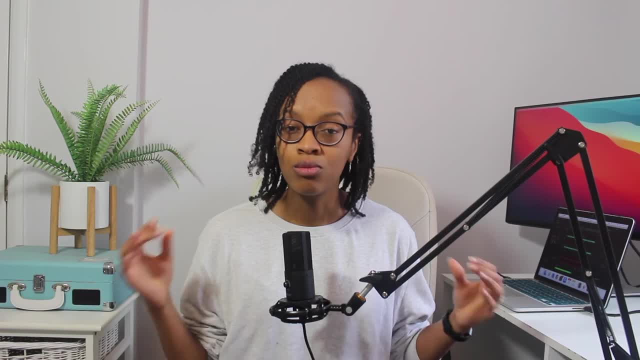 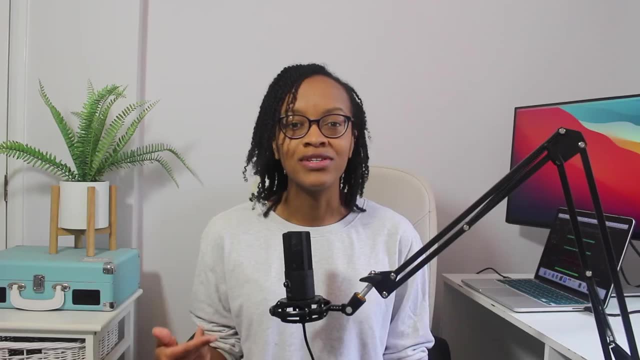 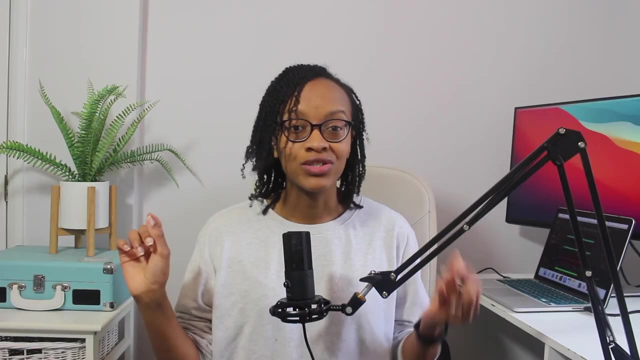 phase of the design process. There are four broad steps in this design process, starting with step one: research. Gather research and develop an understanding through analysis. Step two: design: Ideate solutions from sketches all the way to high-fidelity prototypes. 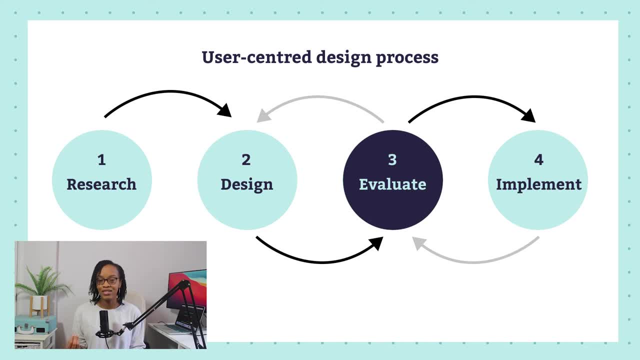 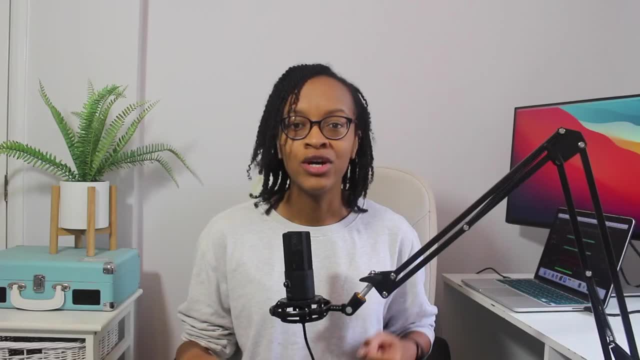 Step three: evaluate. Test your prototypes with users to gain feedback. If further work is needed, you can loop back and iterate on your design, returning to test and gain more feedback. You may need to go through a few iterations before you have a 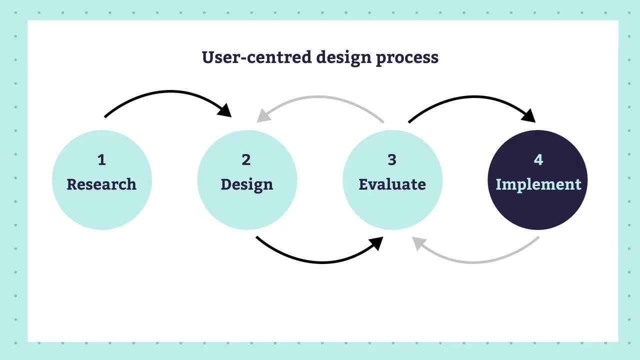 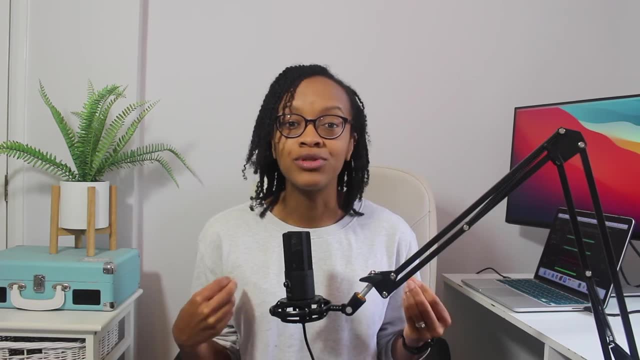 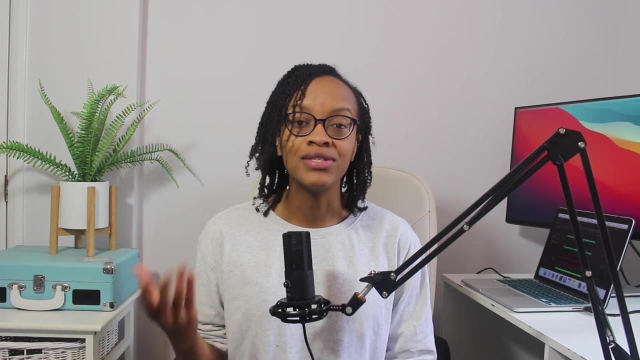 design that users respond well to. Then you can implement your design, Make the feature or website live, monitor analytics and perhaps do further user research, which will take you back to the start of this iterative design process. By using an iterative design process, the product 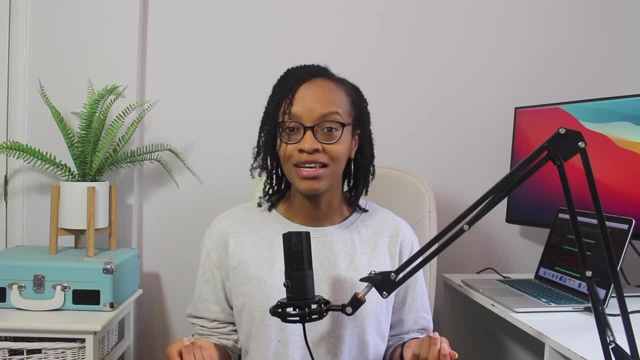 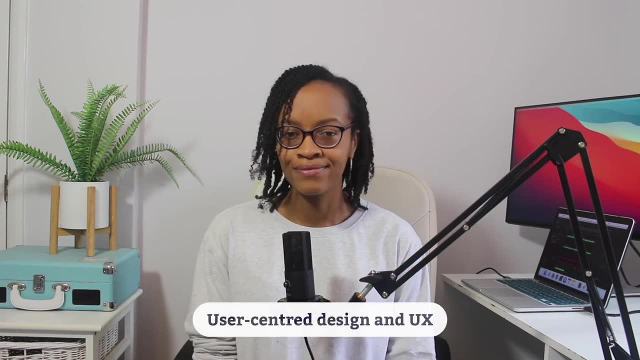 team are constantly working on improving the user experience. It introduces changes gradually and they gain more understanding about their target audience. User-centred design, as mentioned earlier, is a collection of processes which focus on putting the user at the centre of the design. 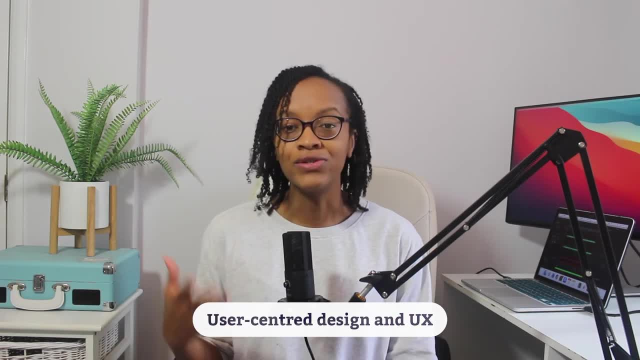 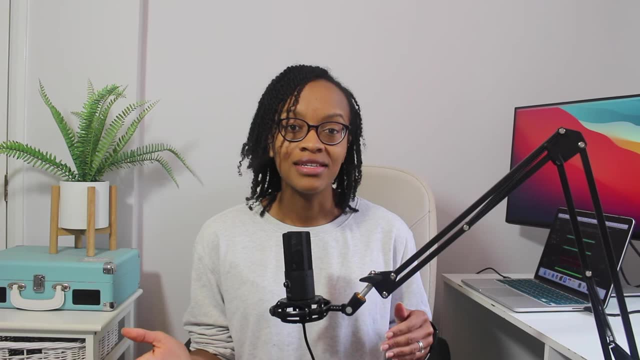 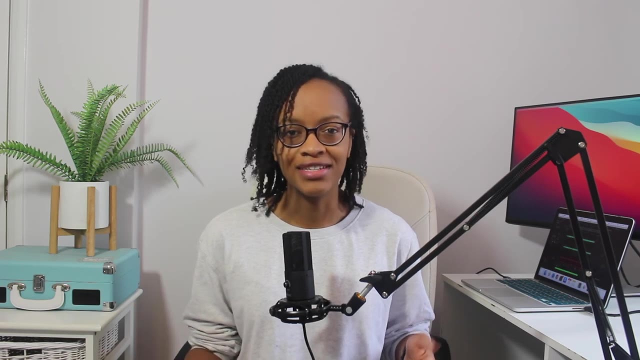 User experience refers to the specific experience users have with the product they use. UX is not necessarily user-centred design. UX is a value of user-centred design, and you need both to create digital experiences that engage your users and meet their needs, If you're not already. 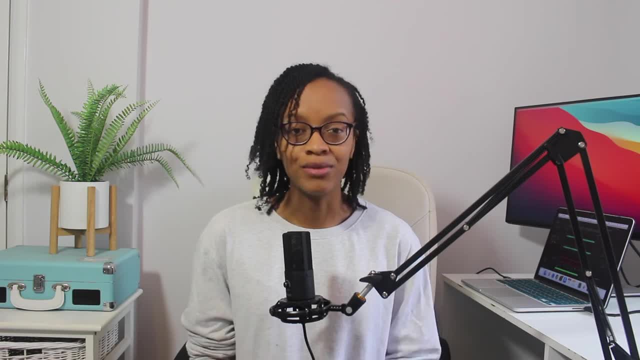 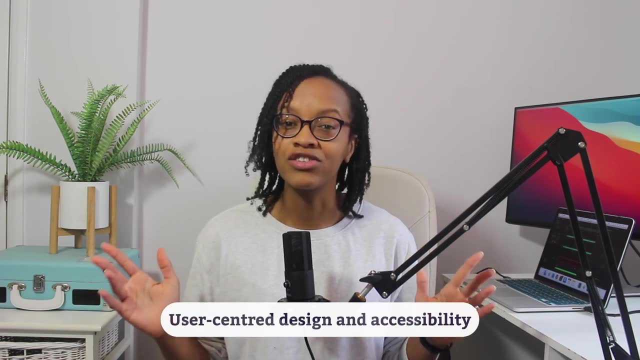 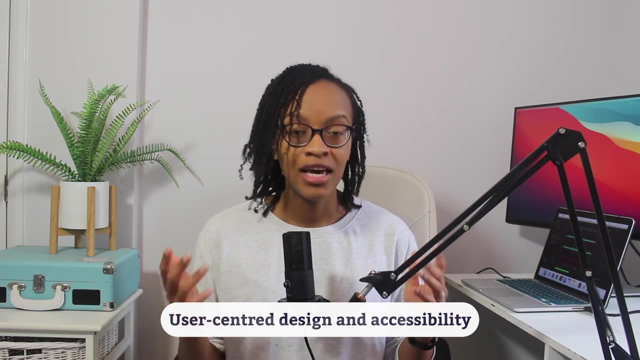 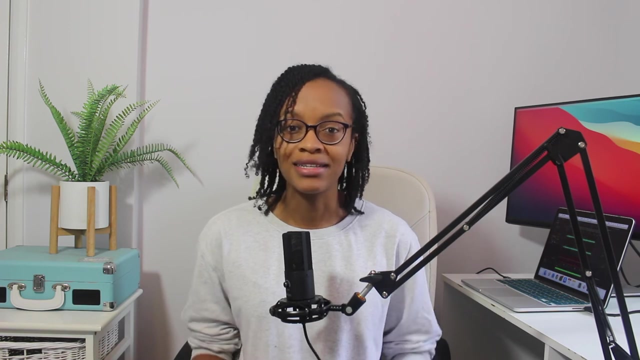 you should definitely be including your users in your design process. Incorporating accessibility into UCD means designers are including the widest range of possible users and situations. User-centred design is a process for designing usable products and user interface. accessibility can be approached as a subset of usability. If you're wanting to learn more about accessibility,